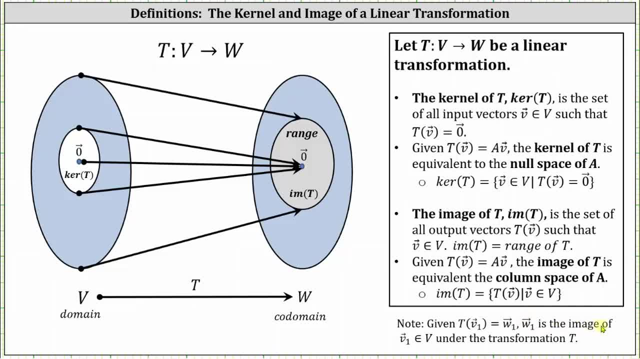 w1. we say vector w1 is the image of the vector v1 under the transformation t. but notice, here we're referring to the image of a single vector. but when we talk about the image of t above, we're talking about the image of the entire transformation. let's take a look at a couple of examples. here we're 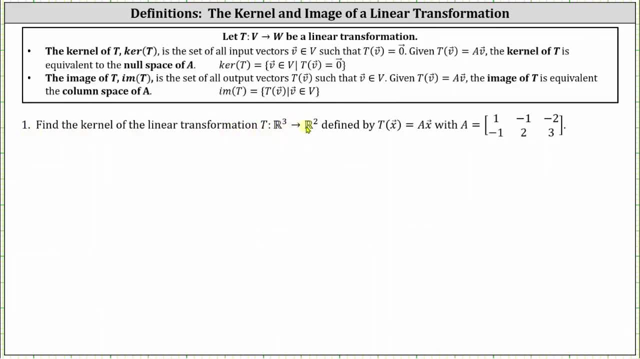 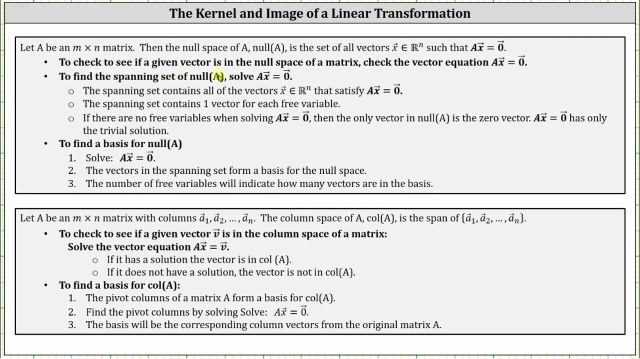 asked to find the kernel of the transformation t from r3 to r2, defined by t of vector x equals matrix a times vector x, with the given matrix a. remember this is equivalent to determining the null space of matrix a. so for a quick review to find the spanning set of the null space of a. matrix. we solve matrix x, matrix a, matrix x, matrix x, matrix y, matrix x, matrix, a matrix and weチャンネル, the spanning set of the null space of a matrix. weaw. we solve matrix double x. we note the spanned space of a matrix and nouvelle germ of the null space of the matrix. we solve matrix, one of the functions of the. 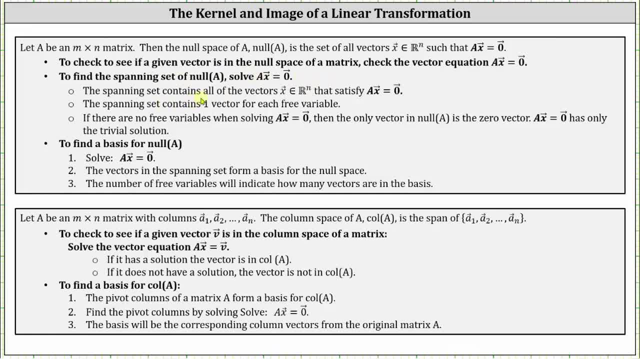 matrix A times vector X equals a zero vector. the spanning set contains all the vectors X in our N that satisfy the equation. The spanning set contains one vector for each free variable. If there are no free variables when solving the equation, then the only vector in the null space of matrix A 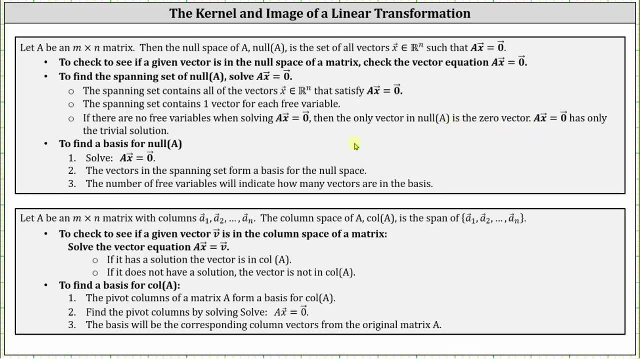 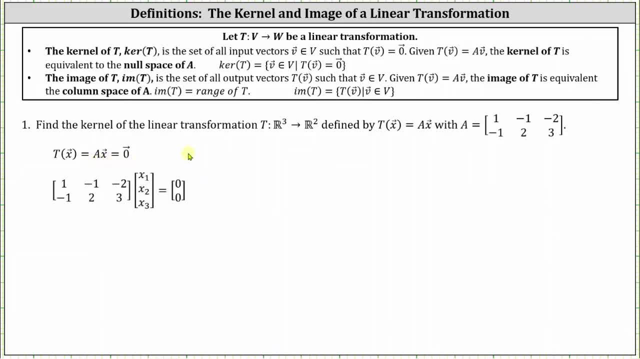 or the image of T, is the zero vector. So, going back to our example, we begin by setting up the equation matrix: A times vector X equals the zero vector, Because we're mapping from R3 to R2, we know the input vector is in R3. 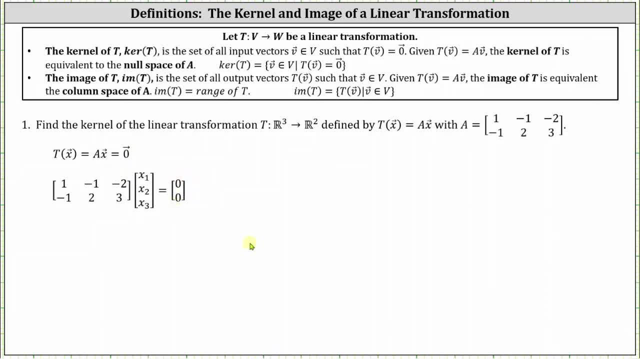 and the output vector. the zero vector is in R2.. This should look familiar. The next step is to set up an augmented matrix and then write the augmented matrix in reducer echelon form. So here we have the augmented matrix, and here we have the augmented matrix. 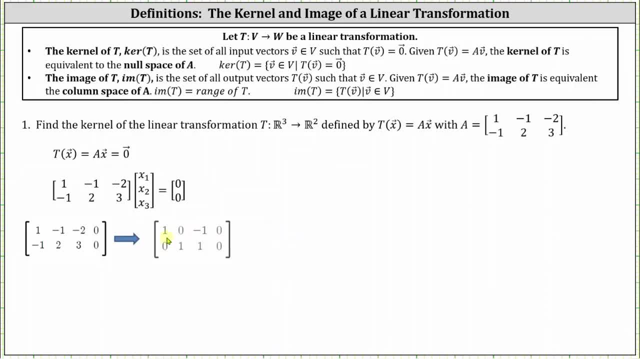 in reducer echelon form. Notice how we have a pivot in column one and column two, but not column three, because we have one free variable. There'll be one vector in the spanning set that makes up the null space of matrix A, as well as the image of T. 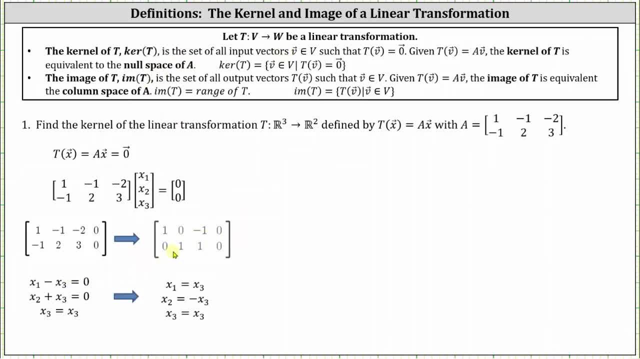 Row one indicates that X1 minus X3 equals zero. Row two indicates X2 plus X3 equals zero And because X3 is a free variable, we know X3 equals X3.. The next step is to solve X1 and X2. 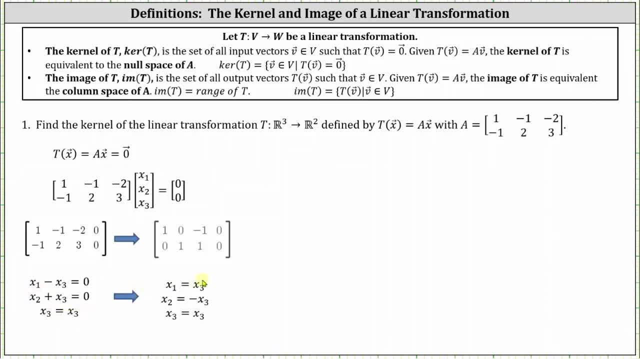 in terms of the free variable X3.. X1 equals X3,, X2 equals negative X3, and X3 equals X3.. Let's parameterize the solution by letting X3 equal T, which gives us the solution. vector X equals T, negative TT. 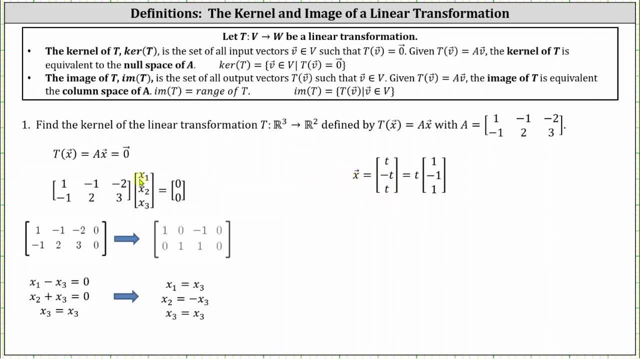 Factoring out the T, we have vector X, which again is the solution to AX. equals zero, is T times the vector one negative one one. So now we know, the kernel of T, which is also the null space of matrix A, equals the span of the vector one negative one one. 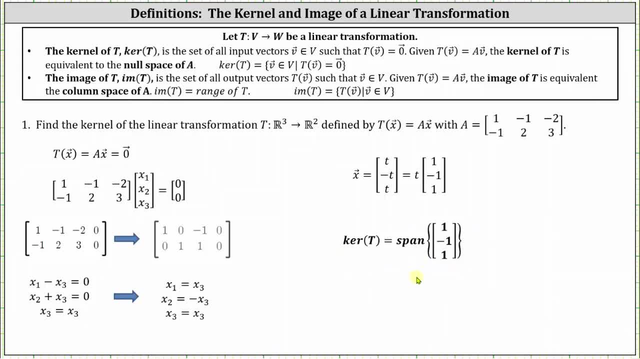 So, because we only have one vector in the span, all the linear combinations of this vector give us all the vectors in the domain of the transformation T that map to the zero vector or have an output vector of zero. And now for the second example. 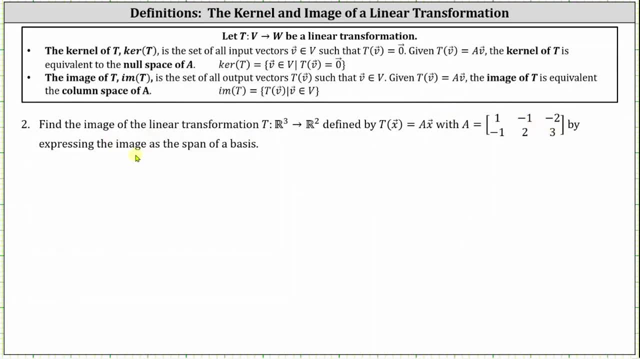 let's find the image of the same linear transformation by expressing the image as the span of a basis. Remember, this is the same as expressing the column space of matrix A as a span of a basis. So, for a quick review, the pivot columns of matrix A form a basis. 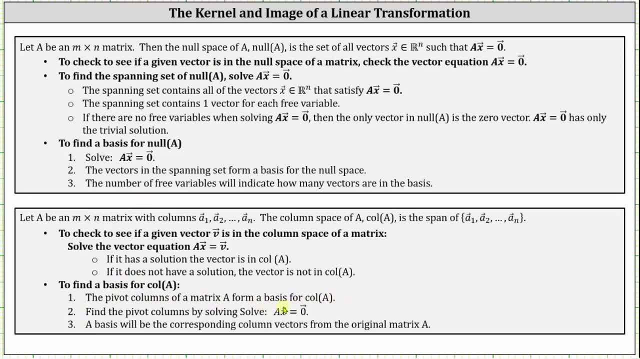 for the column space as well as the image of T. We find the pivot columns by solving the same matrix equation. matrix A times vector X equals a zero vector. A basis will be the corresponding column vectors from the original matrix A, And once we have a basis, 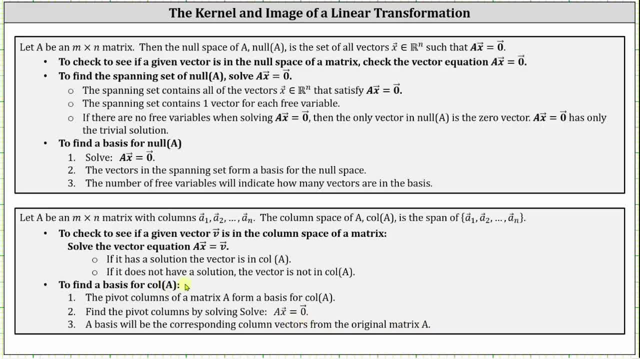 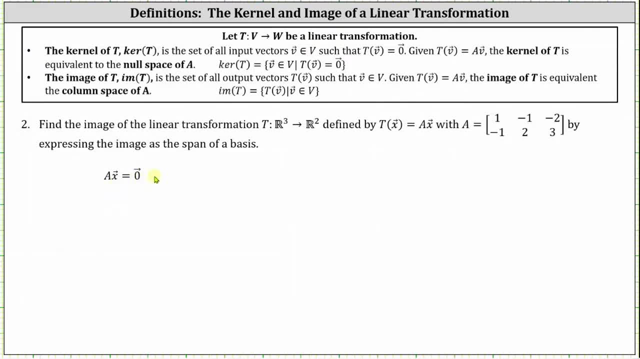 we can express the column space of matrix A as well as the image of T as a span of the basis. So again, we set up the equation: matrix A times vector X equals a zero vector, which we already did in the previous example. 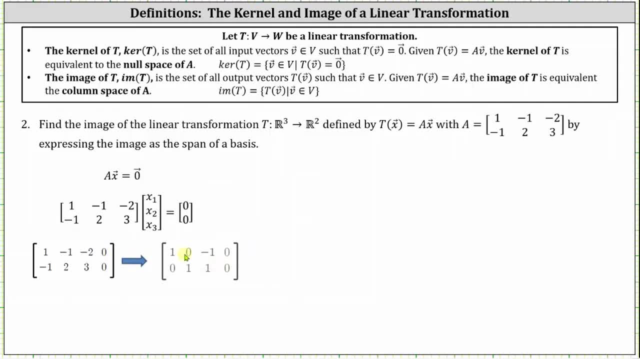 then write the augmented matrix in reduced echelon form. But here's where our work changes. The next step here is to identify the pivots. We have a pivot in row one, column one, as well as row two, column two. or we have pivots in column one and column two. 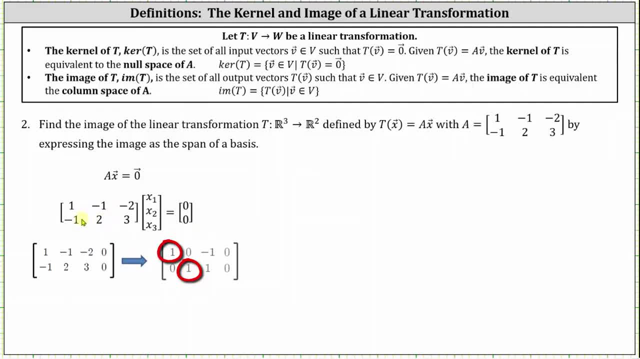 which means column one and column two of the original matrix A form a basis for the image of T as well as the column space of A. So again now we know a basis for the column space of A as well as a basis for the image of T. 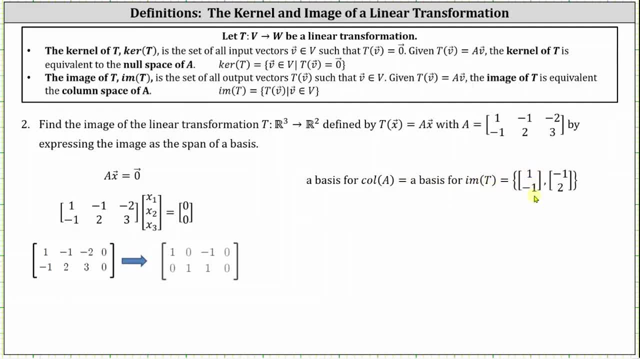 is equal to the set containing the vectors one, negative one and negative one, two, and therefore the image of T equals the span of the set containing these two vectors, which indicates all the linear combinations of these two vectors will give us all the output vectors. 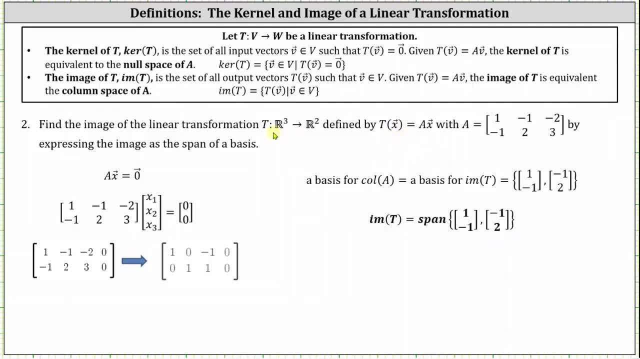 T of vector X. given vector X is in the domain or in R3.. I hope you found this helpful.